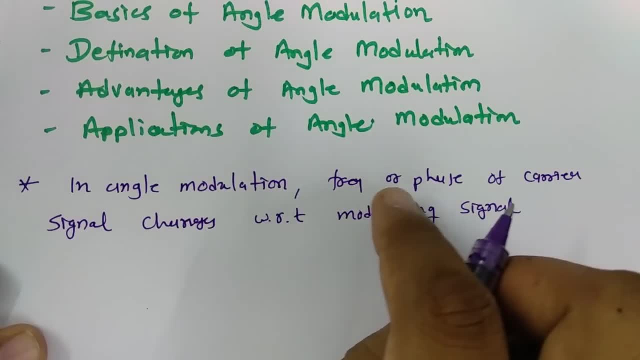 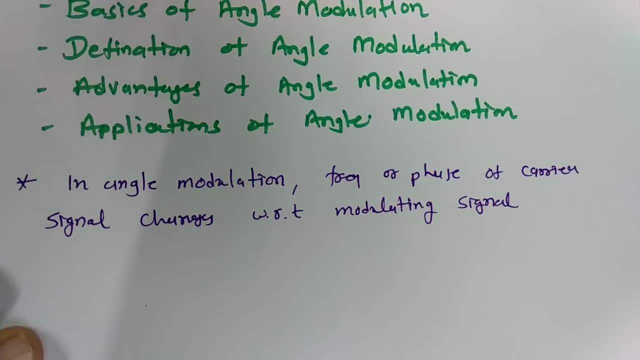 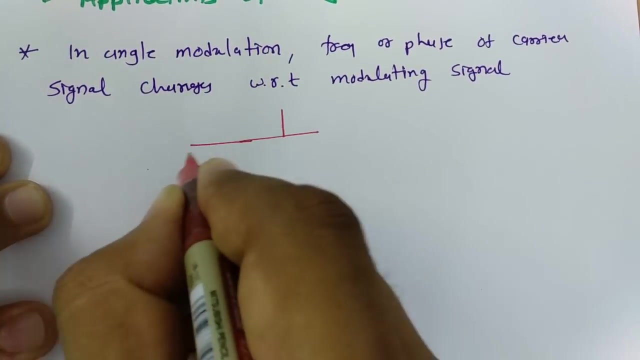 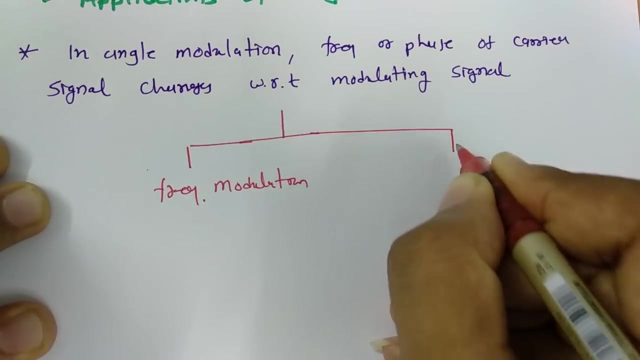 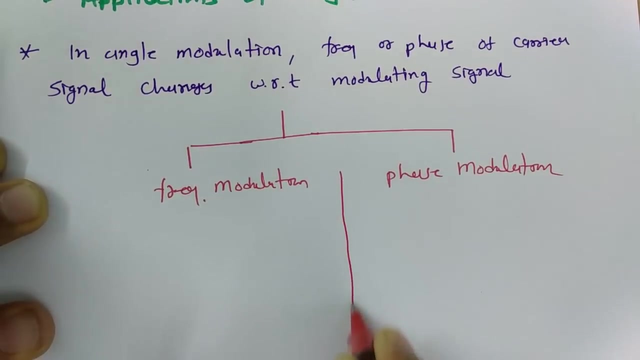 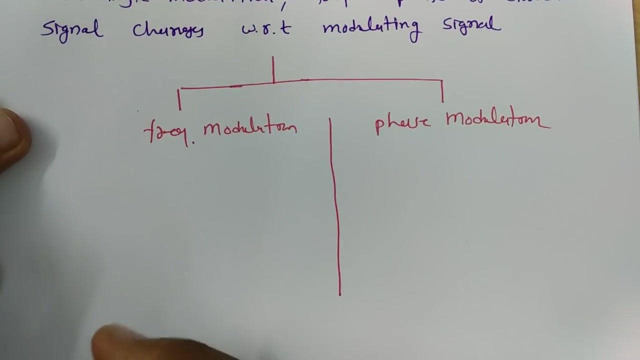 we talk about angle modulation, Where what we do is we change frequency or phase of carrier signal with respect to modulating signal. So basically, angle modulation that is classified in two parts: One is frequency modulation and second part that is phase modulation. So what is frequency modulation? So when we talk about frequency modulation, in which frequency of 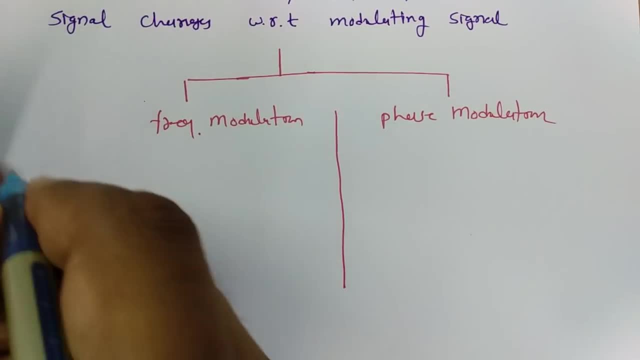 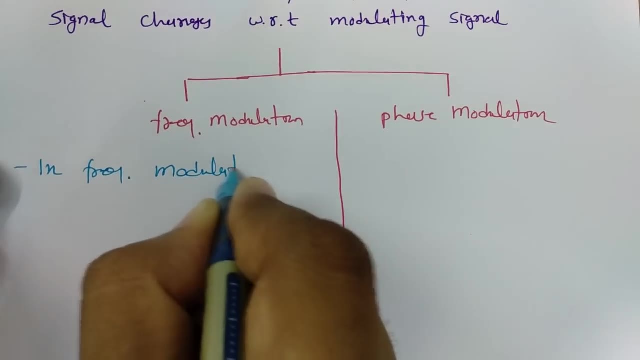 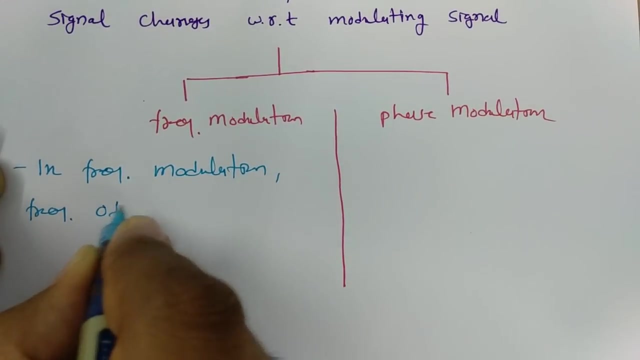 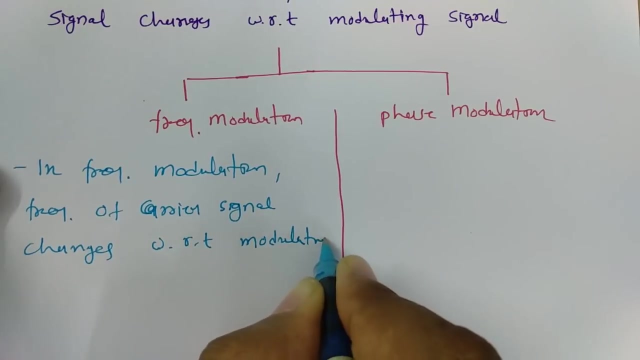 carrier signal changes with respect to modulating signal. So in frequency modulation frequency of carrier signal changes with respect to modulating signal. So what is frequency modulation changes with respect to modulating signal? So as if I say we have carrier signal Ct. 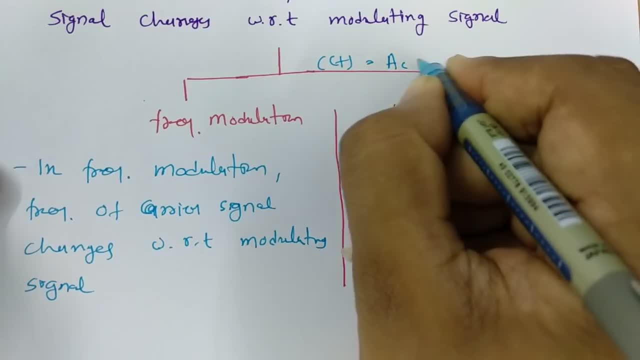 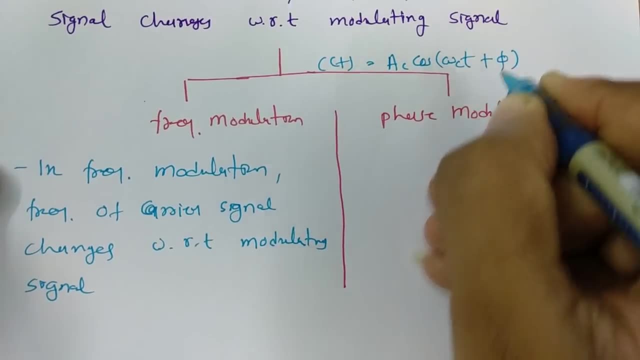 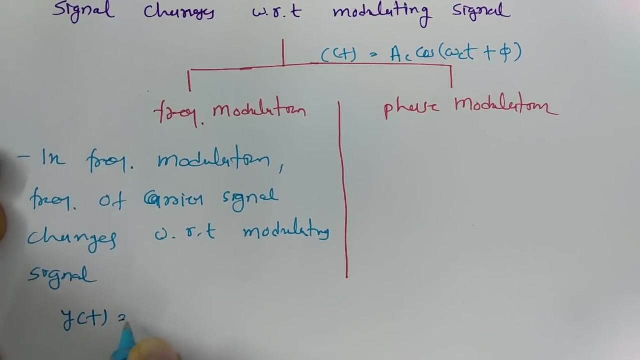 and that is Ac cos omega, Ct plus phi. So in that frequency modulation my output signal that has to be having constant amplitude. So amplitude will be as it is. cos of now I will be writing omega of T plus phi, where this omega of T that will be function of modulating signal. So omega of T. 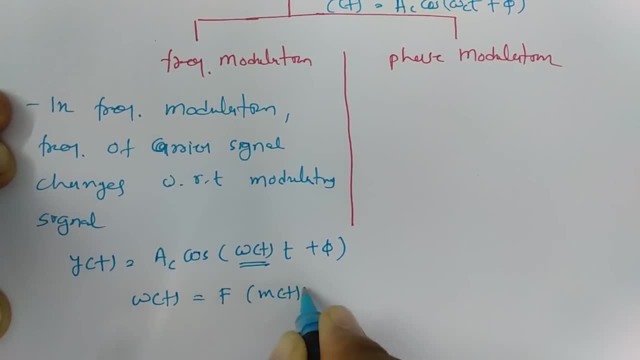 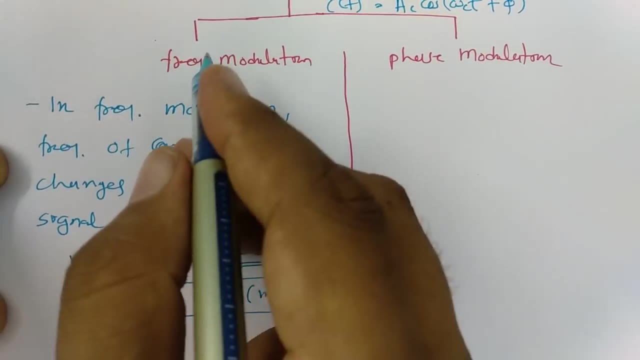 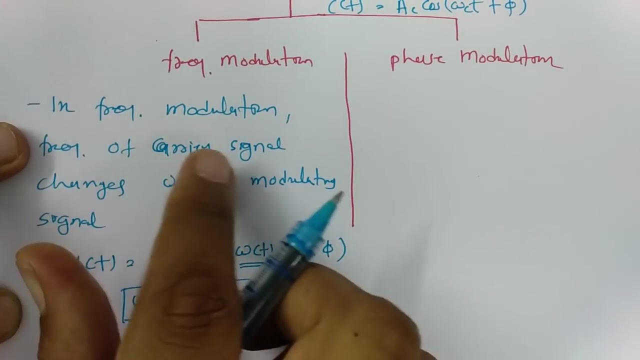 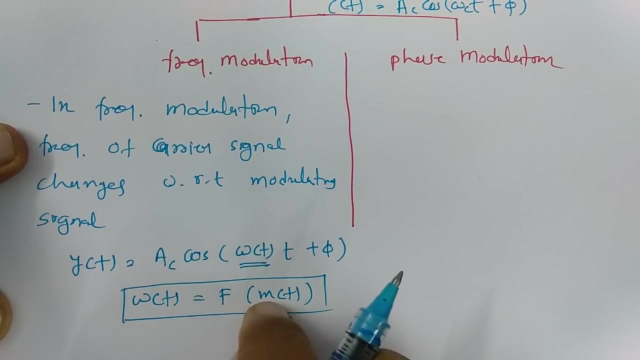 that will be function of modulating signal and that is how carrier signal will change and that is what will be sending over frequency modulation. So frequency modulation is a process in which frequency of carrier signal changes with respect to modulating signal signal. So here, frequency of carrier signal, that is getting changed as a function of modulating. 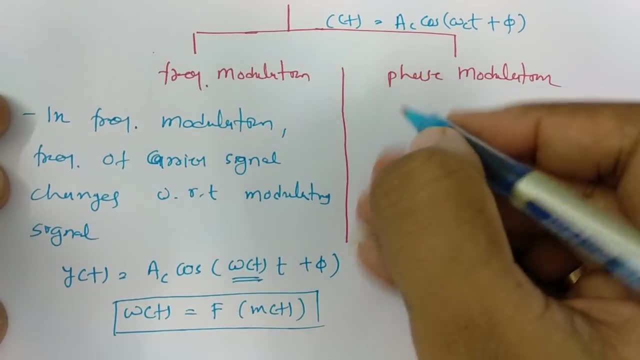 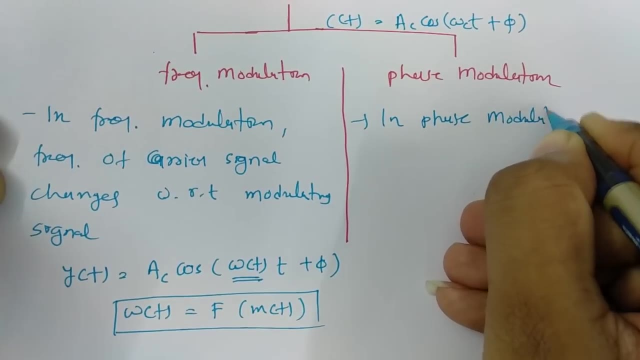 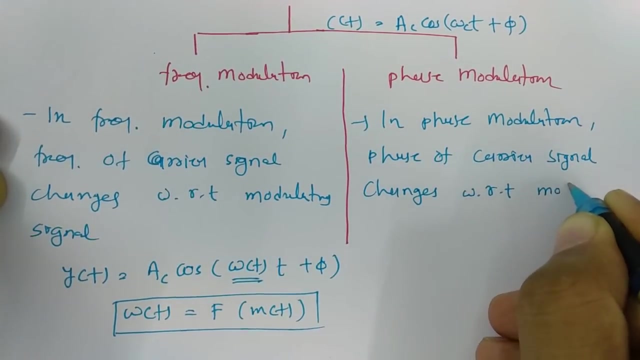 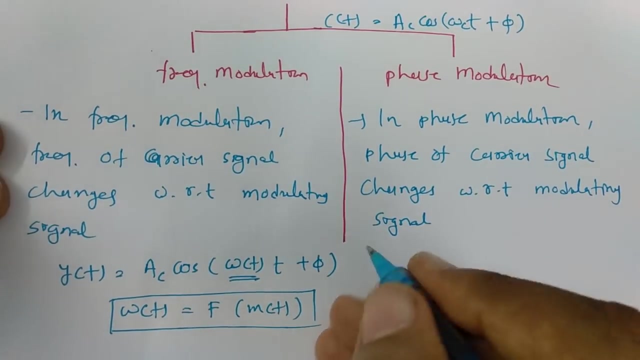 signal. that is what frequency modulation. Now when we talk about phase modulation. so in phase modulation phase of carrier signal changes with respect to modulating signal. So if I want to explain you function, then that function function would be yt- modulating yt. 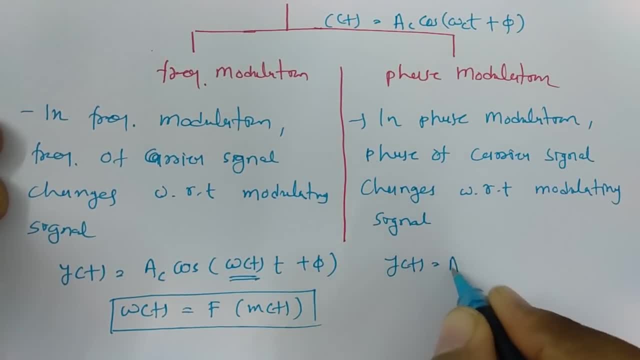 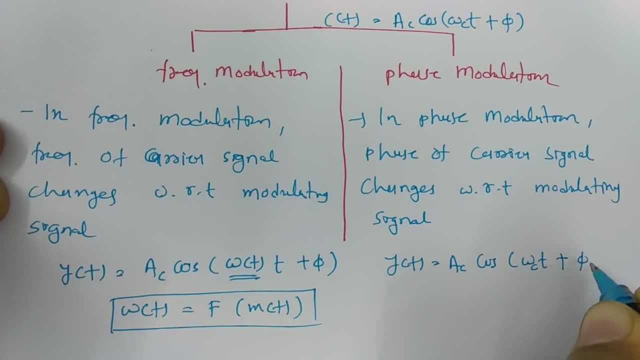 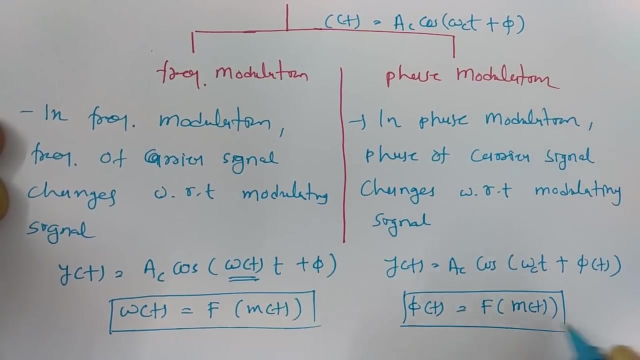 where carrier amplitude will remain constant. So AC cos of frequency 1 will be constant. So it will be omega c t plus now phi. that will change with respect to modulating signals. I am writing it as phi t, where phi of t that will be function of modulating signal m t. So here phi t is changing. 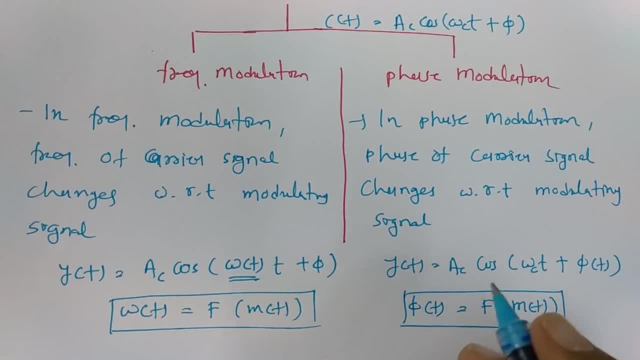 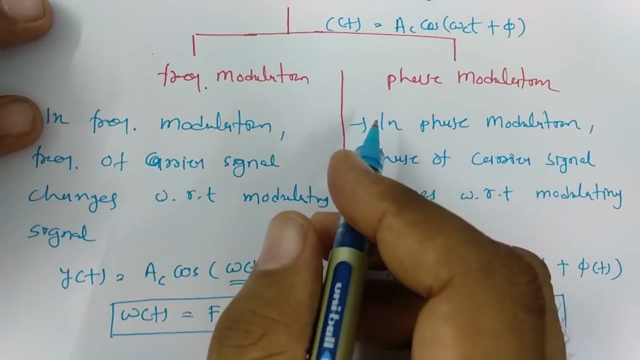 with respect to modulating signal and carrier signals. phase, that is what. changing with respect to modulating signal, that is what phase modulation And combination of frequency modulation and phase modulation, that is what we say it as angle modulation. So this is what angle modulation. 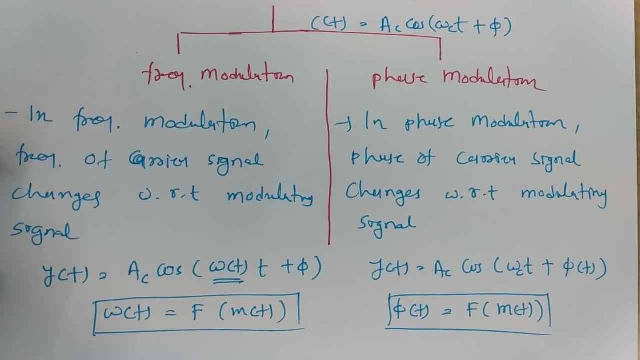 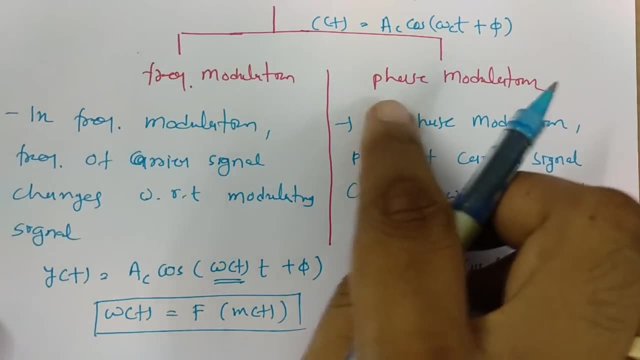 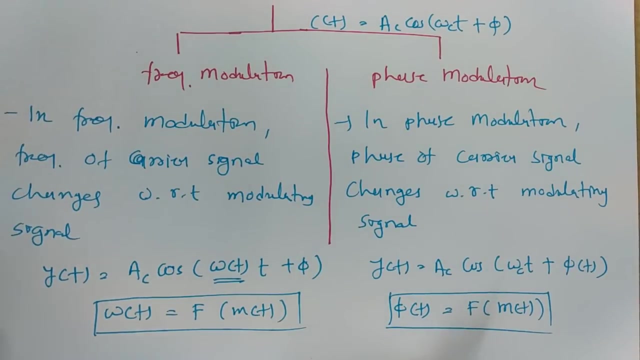 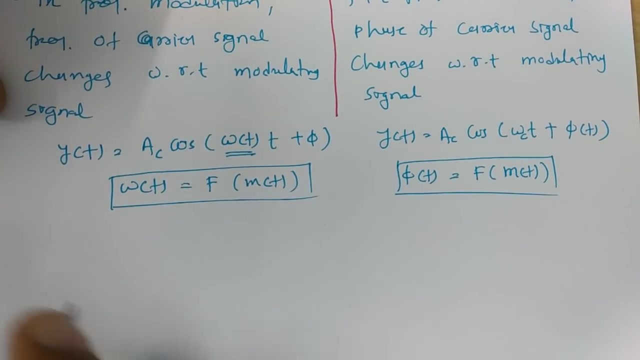 So angle modulation means frequency modulation or phase modulation. In frequency modulation we change frequency of carrier signal with respect to modulation, And in phase modulation we change phase of carrier signal with respect to modulating signal. Now let us discuss few advantages of angle modulation. 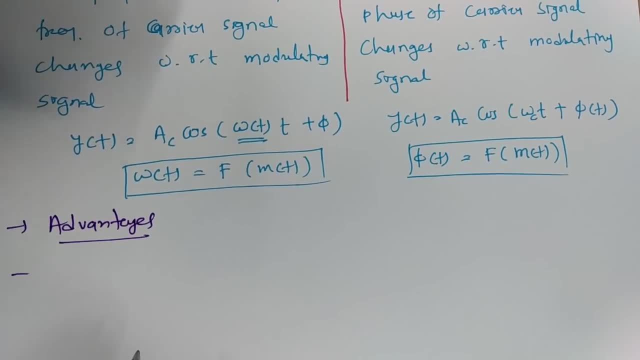 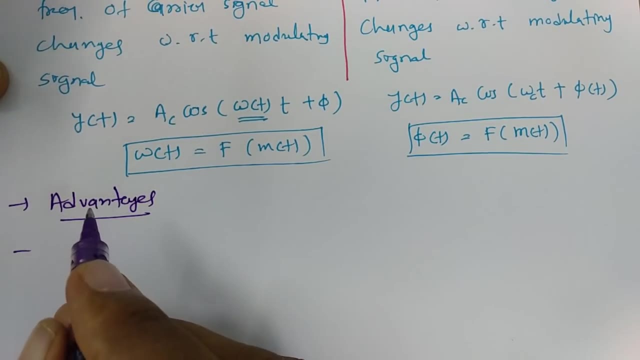 So we have seen already amplitude modulation in my previous videos. you can see those videos where We have some advantages of angle modulation over phase modulation, sorry, angle modulation over amplitude modulation that I will be discussing here. One is noise reduction. Why noise reduction is happening? The reason is in AM, our carrier signals, amplitude is changing. 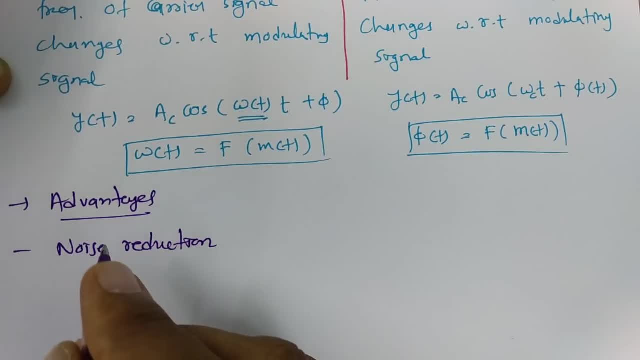 with respect to modulating signal, where here amplitude is remaining constant, here phase or frequency is changing. So there will be always advantage when we work with frequency over phase, rather to work out with amplitude. The reason is, when you send signal with variation of amplitude by antenna because of noise, maximum affection, maximum defect, that will happen with amplitude, only minimum defect, that happens with frequency. So in phase modulation noise reduction is happening. 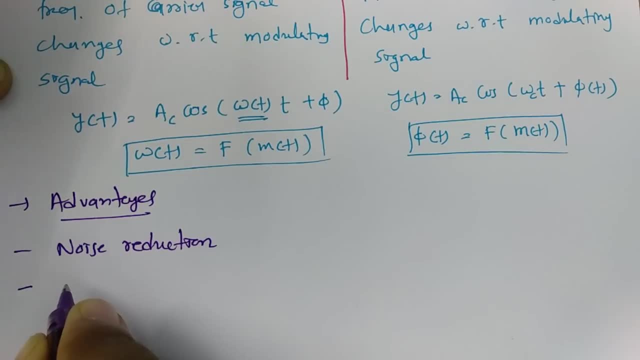 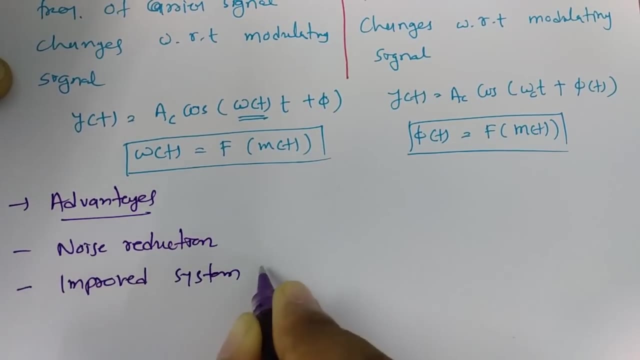 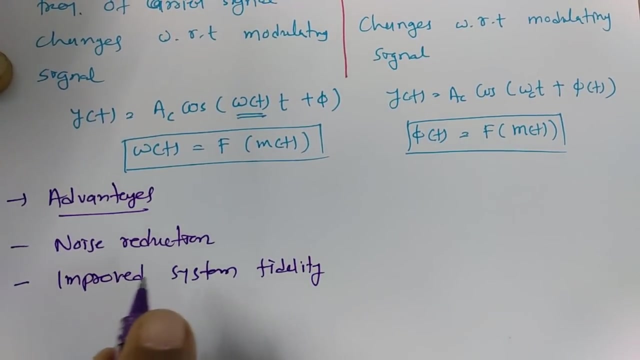 Second basic advantage, that is Improved system feedability, So improved System Fidelity. So when you have multi path fading, even in that case even we will be having improved system fidelity. So that is one basic advantage and most important advantage, that is efficient use of power. 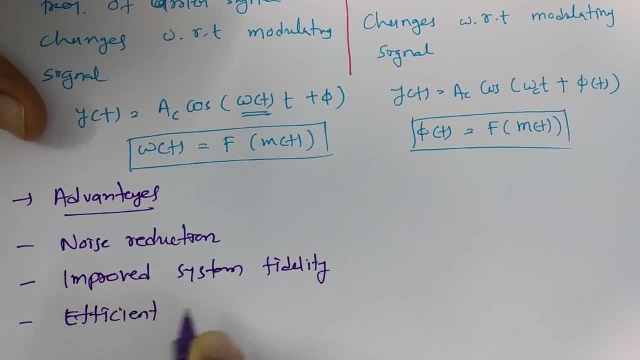 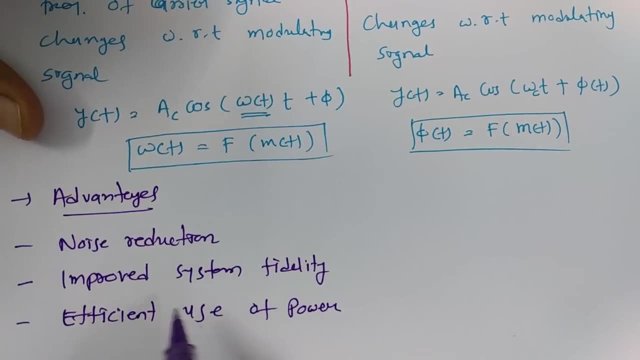 So that is one basic advantage and most important advantage, that is, efficient use of power. if you see amplitude modulation, then we have been sending carrier signal in that and that carrier signal is having maximum power, while in case of angle modulation we don't send separate carrier signal, we have only modulated signal and that is having entire power. so 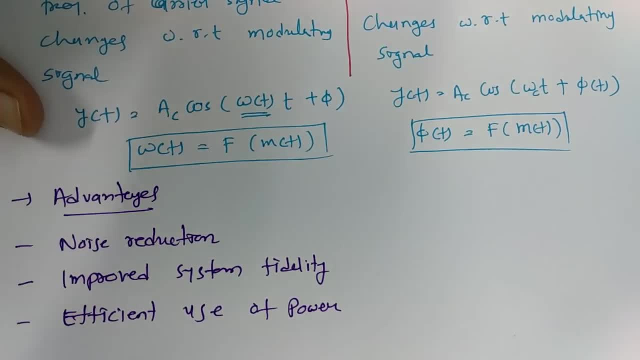 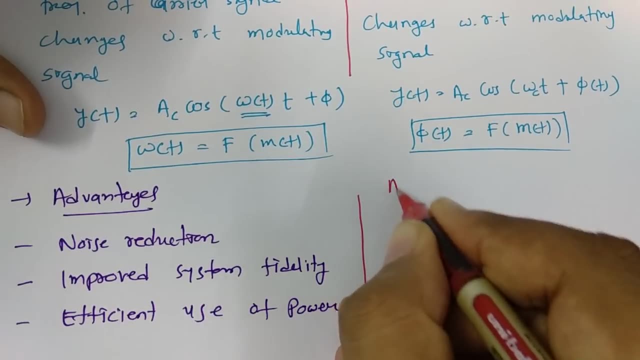 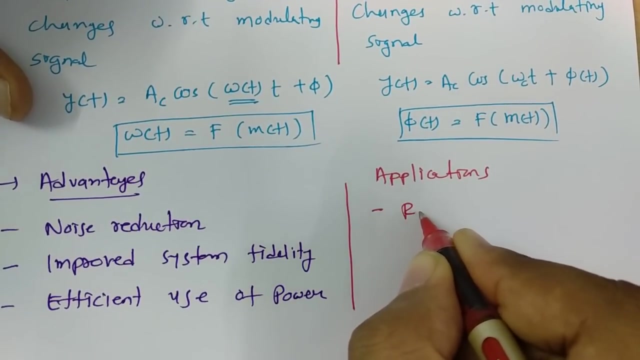 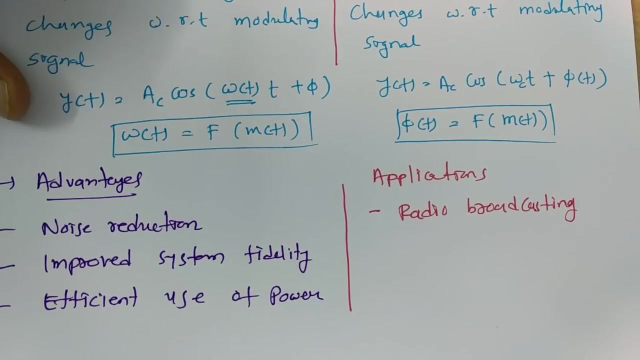 efficient use of power. that is happening in angle modulation. Now let us discuss few applications. so basically we use this in radio broadcasting. you can see FM, which is what we are receiving right now. in India, frequency ranges from 88 megahertz toci Magbyp. this has been used for broadcasting on TV shows of maximum current. frequency ranges from 88 megahertz to 快速迴顶. crises far away at kneading villages. so this is what our renders: A1 wie divert function, SNR W use this as fascia of波線. it does not by default. 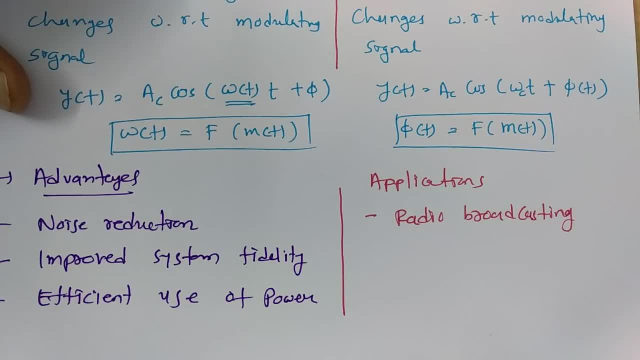 to 108 megahertz. that is what happening with frequency modulation, so radio broadcasting that we can do it. second is TV sound transmission. TV sound transmission, so sound carrier, that is what we are modulating it by frequency modulation in TV sound transmission. cellular radio, that is even one. 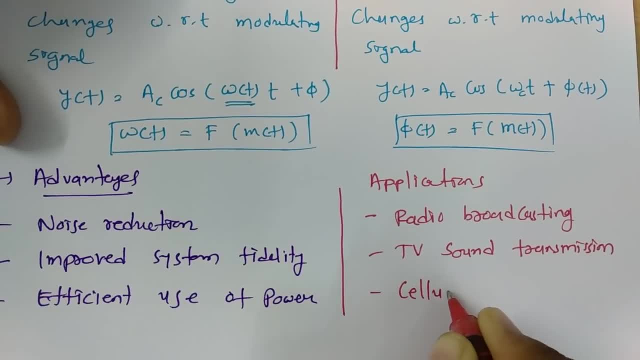 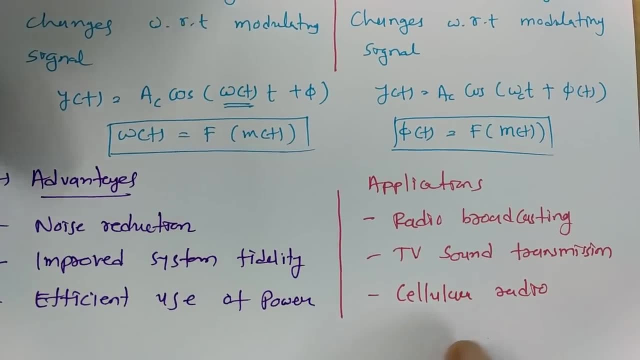 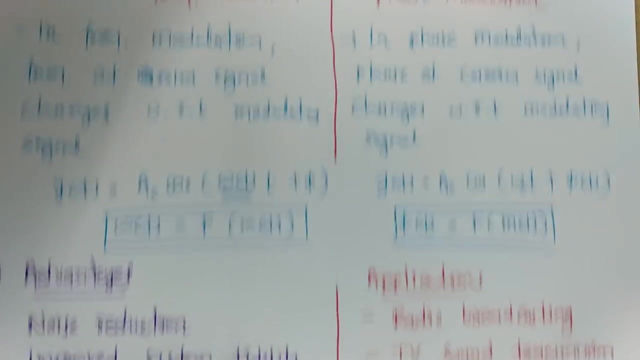 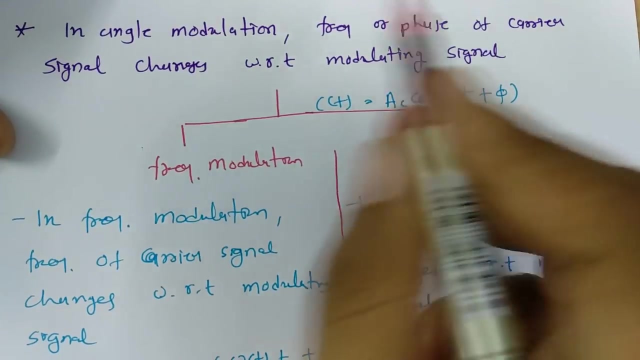 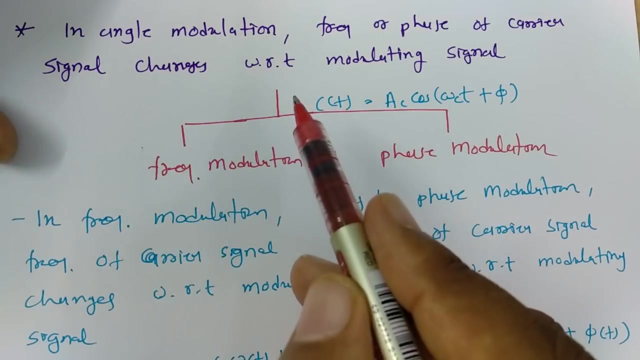 important application. so these are the basic applications, which is what we are using it in angle modulation. so let us have brief again. what is angle modulation? in angle modulation, frequency or phase of carrier signal changes with respect to modulating signal. so basically, angle modulation that is classified in two parts: frequency. 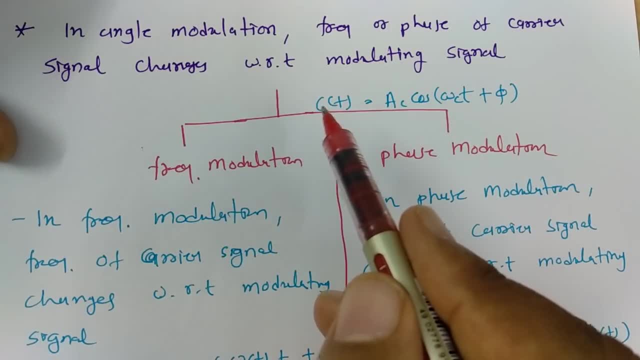 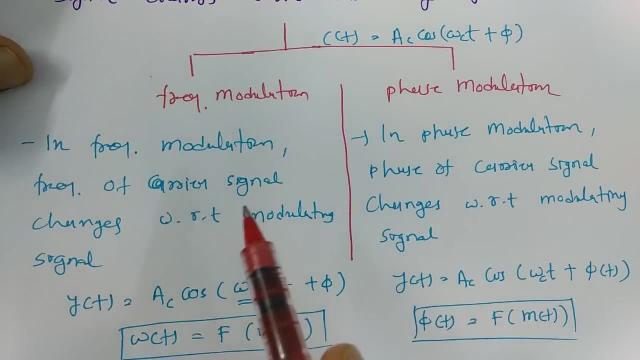 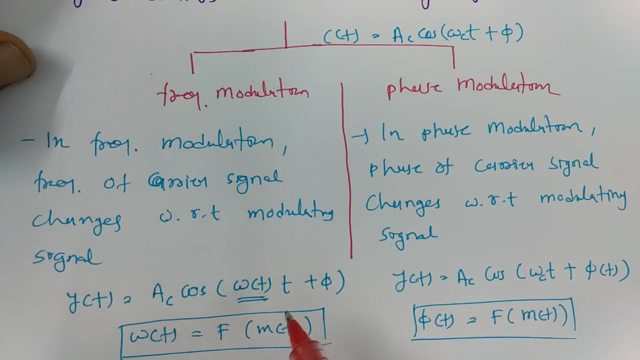 modulation, phase modulation. if I say my carrier signal is CT, that is equals to AC, cos, Omega, C, T plus 5, then in frequency modulation, frequency of carrier signal, that is changing with respect to modulating signal. so frequency of modulated signal will be function of modulating signal. 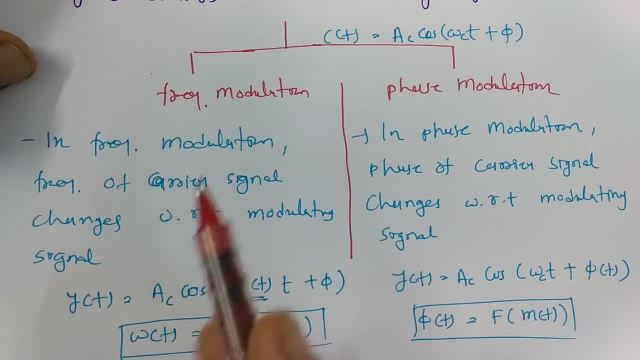 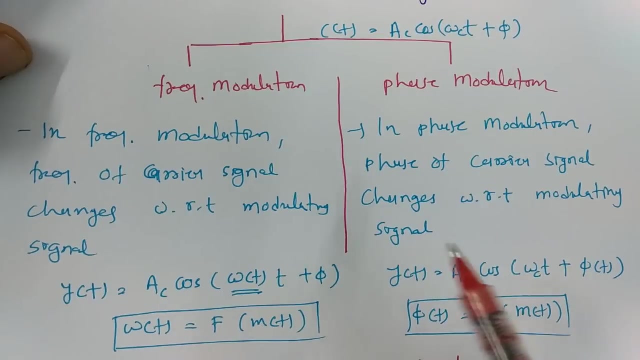 so my modulated signal by frequency modulation, that will be AC cos of Omega T as a function of modulating signal, T plus 5, while in case of phase modulation we change phase of carrier signal with respect to modulating signal. where we change phase with respect to modulating signal, so phase will be function of 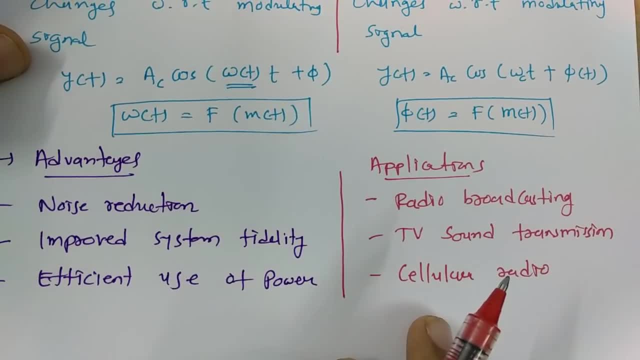 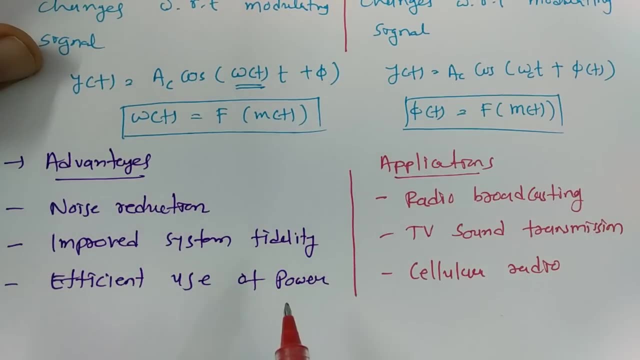 modulating signal. we use this angle modulation because of so many advantages over amplitude modulation, like noise reduction, improved system fidelity, efficient use of power. so these are the major advantages. that is why we are using angle modulation, and applications are radio broadcasting, TV, sound transmission and cellular radio. so this is how we have angle modulation in. 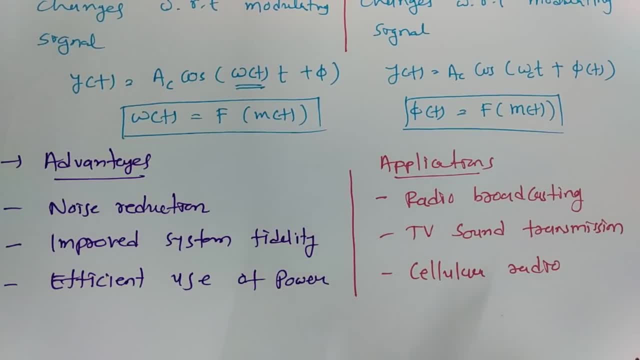 detail explanation of frequency modulation and phase modulation. I'll be making next few videos, so just stay tuned with this channel. you will be finding complete detail of frequency modulation and phase modulation, and even I will solve few problems. that will explains you clear idea about how we can utilize